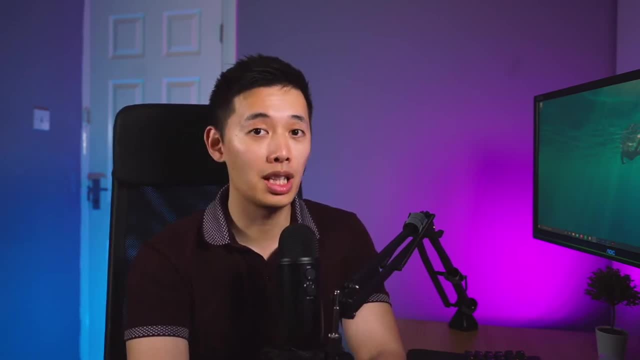 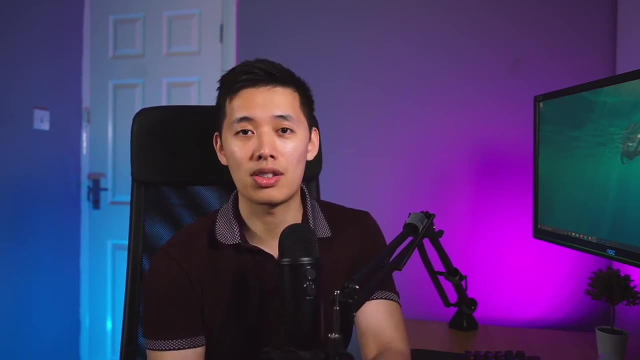 would be XGBoost. that's already helped win a lot of Kaggle competitions. And before you can understand how these algorithms work, you need to understand the difference between decision trees, random forests and also gradient boosting. So here are the timestamps in case you want to skip. 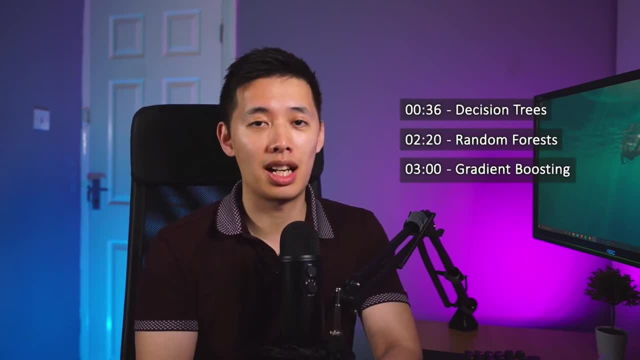 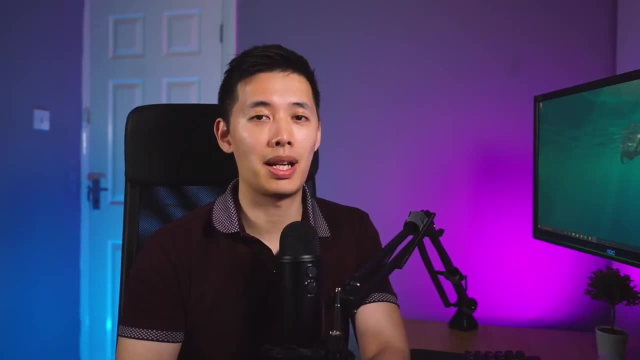 ahead. In this video, I'm going to go over at a high level what the differences are, because even sometimes I forget. Let's get right into it. So decision trees are very, very simple predictors. Basically, they represent a series of conditional steps that you need to take in order to make a 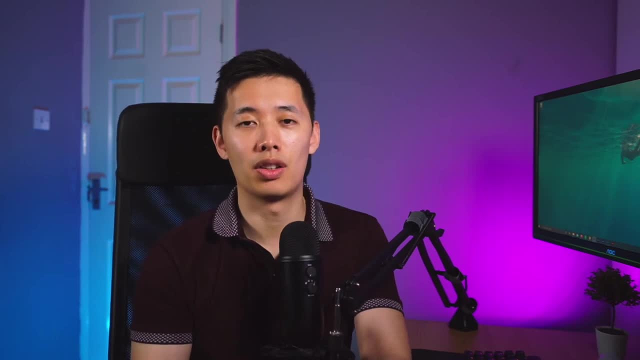 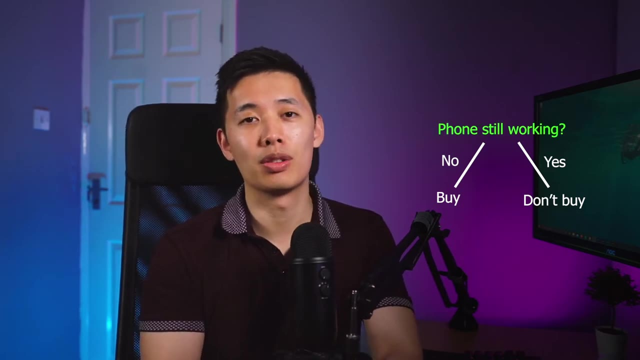 decision. As a very basic example, let's say I'm trying to decide whether or not it's worth buying a new phone, And I have this very simple decision tree to help me decide. The first and only question is: does my current phone still work? Well, yes, it does So, according to this decision. 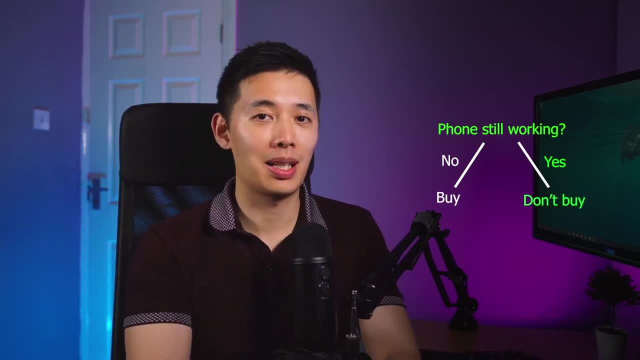 tree. that's a very simple decision tree, So I'm going to go over at a high level what the differences between decision trees are, And that's it. I don't need to buy a new phone Now. would something as simple as this actually be useful in modeling the problem? Probably not, because there's a lot. 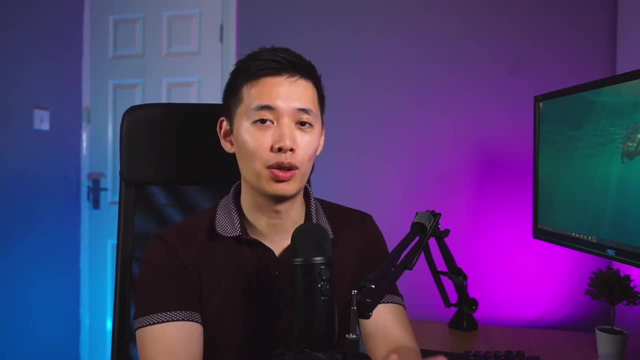 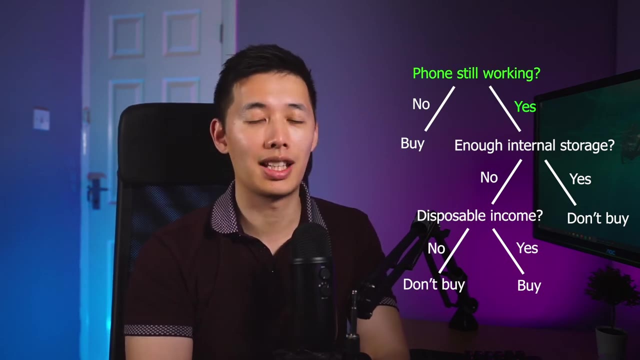 of other factors to take into account than just whether or not my current phone is still working. So instead we can have a more complex decision tree like this one, which asks: does my phone still work, Which yes, it does- Do I still have enough memory capacity to record videos and take? 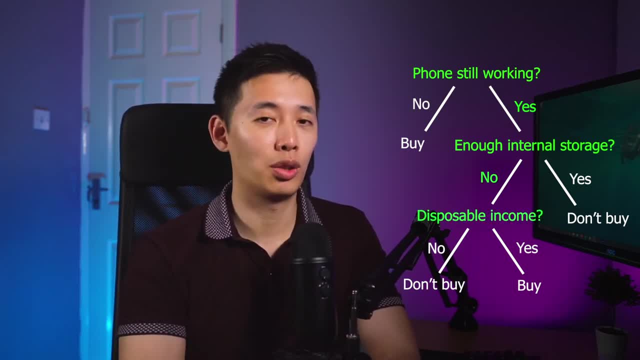 photos? No, not really. Then we move further down. Do I have enough disposable income to buy a new phone? Yeah, I do So, then the decision would be to buy a new phone. So I'm going to go over at a. 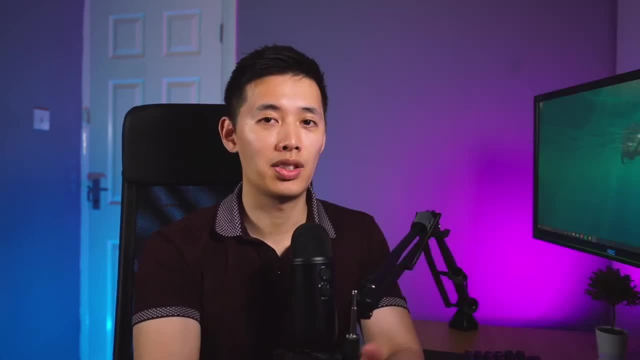 decision tree. Now, in this example you can see that if we wanted to keep going further and further down the tree, we can easily do that just by adding more questions. Or if we wanted to make the tree simpler, then we would just remove some of the questions from the tree. They're very easy. 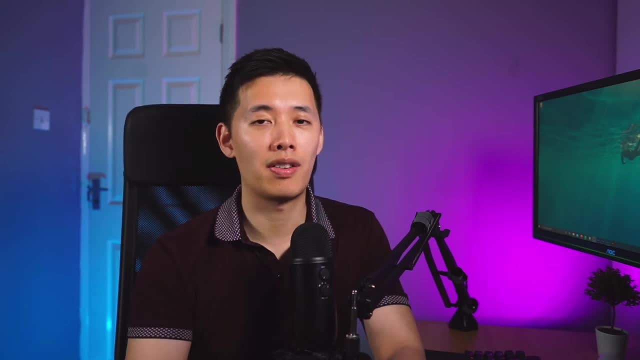 to use and they provide a clear visual for making decisions, And they're also very easy to build computationally as well. However, there's some serious disadvantages to this simplicity, the main one being overfitting. So it performs extremely well on one data set, But if you try to 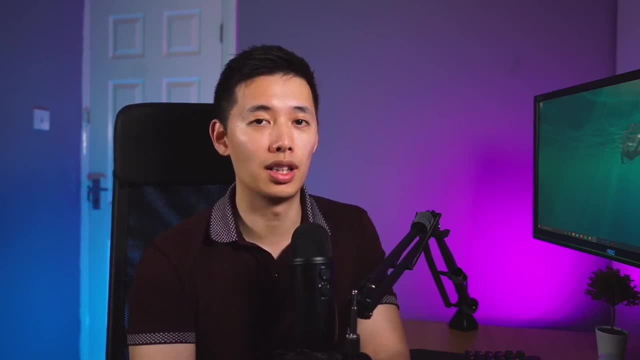 generalize this model on other data sets, you're going to have to go over and over and over and over. less than it performs very poorly. You can see in the example I showed, the further down the tree you go, the more specific that tree becomes for that particular situation. Also, depending on the 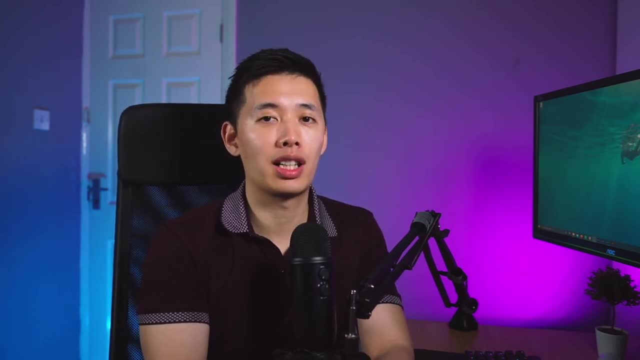 question you start building the decision tree with, the final decision tree can end up looking very different. So in the end, despite them being easy to build, you wouldn't use a decision tree by itself to make generalized predictions with. And this brings us on to random forests Now. 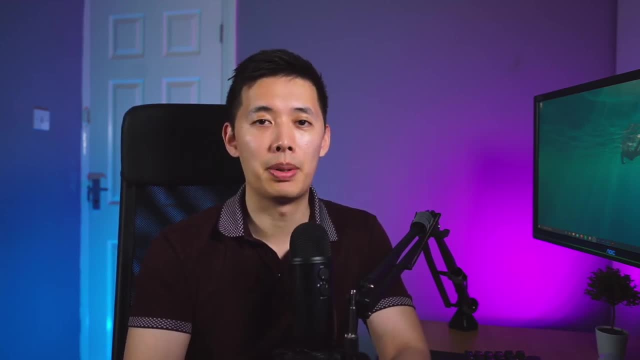 random forests use a concept called collective intelligence. It builds a bunch of decision trees independently, which are simple predictors, and aggregates their results into a single result. This collective result should, in theory, be closer to the true result that we're looking for. As I said earlier, decision trees can look very different depending on the data it uses. 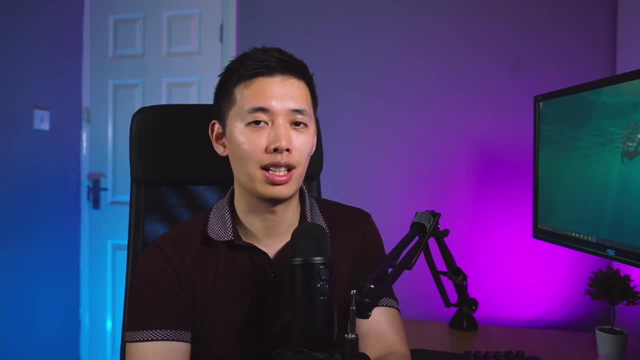 Random forests will try to randomize the construction of trees to try and get a variety of different predictions. However, random forests are harder to interpret because they're a group of decision trees, They're not just a single decision tree anymore And they're also slower. 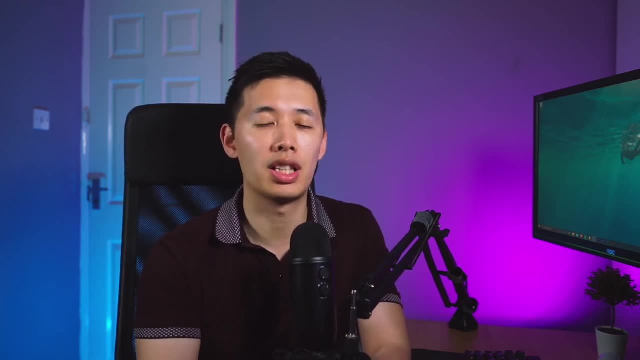 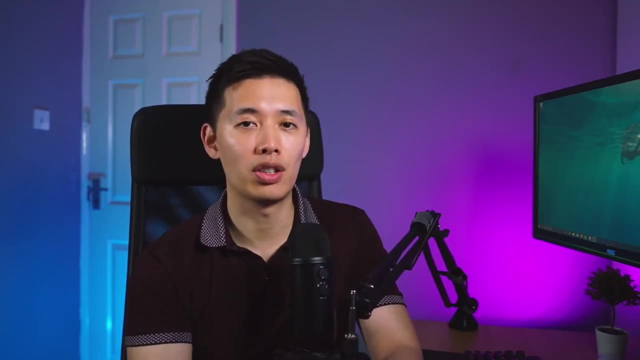 to build, because the algorithm needs to build them. So if you're looking for a decision tree, you build and evaluate each decision tree independently. Now, like random forests, we also have something called gradient boosting, which is also a collection of decision trees. The main difference: 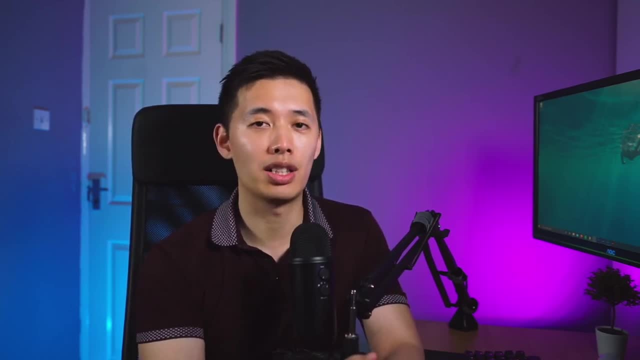 between random forests and gradient boosting lies in how the trees are created and also how they're aggregated. The trees in gradient boosting are built additively, meaning that each tree is built one after another, and each tree is built to improve on the deficiencies of the previous trees. 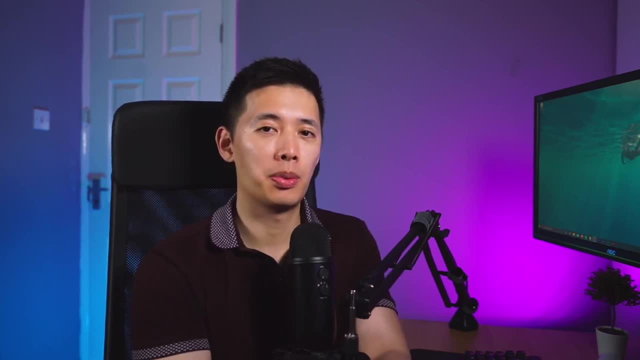 This whole concept is called boosting The gradient. part of gradient boosting comes from minimizing the gradient of the loss function. So if you're looking for a decision tree, you can build one at a time to improve the overall model instead of being built independently. Another key difference between random forests and gradient boosting is how they aggregate the results In gradient boosting. instead of aggregating the results at the end of the process, it aggregates the results along the way to calculate the final result. Overall, gradient boosting usually performs better than random forests, but they're prone to overfitting. 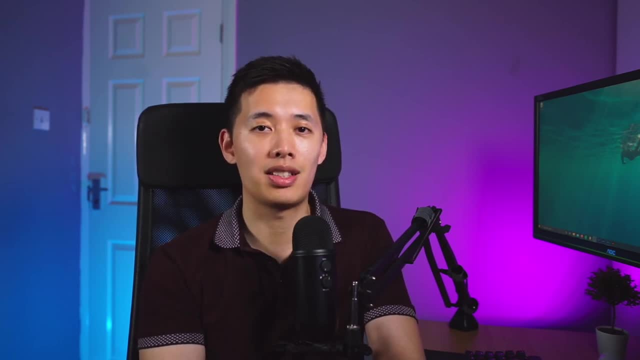 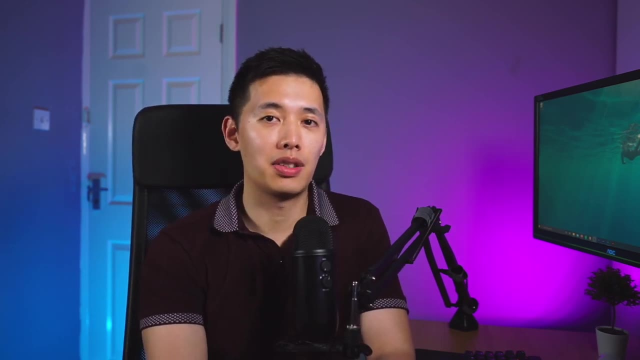 if you don't tune the parameters very carefully. They're also very sensitive to outline, So if you think your data has a lot of noise, then gradient boosting might not do very well. So hopefully this video helps clarify the differences between decision trees. 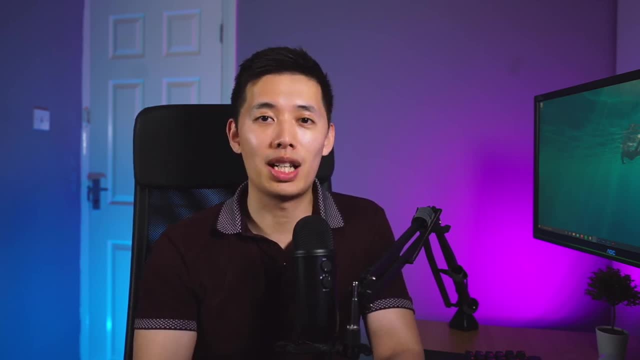 random forests and gradient boosting. Gradient boosting is really popular nowadays, so I think it's worth knowing what the differences are. I've got more beginner data science videos up here somewhere that you can check out as well And if you want to stay updated. 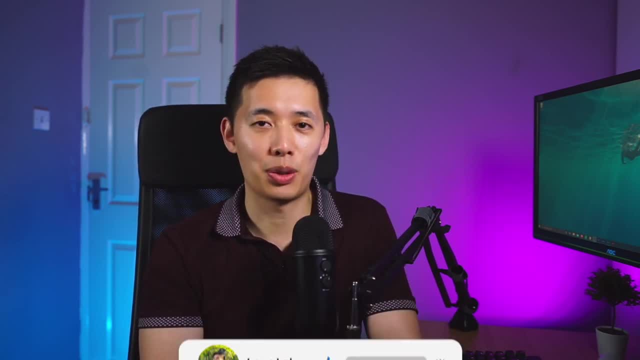 please like and subscribe. turn on the notification bell and I'll see you in the next one.